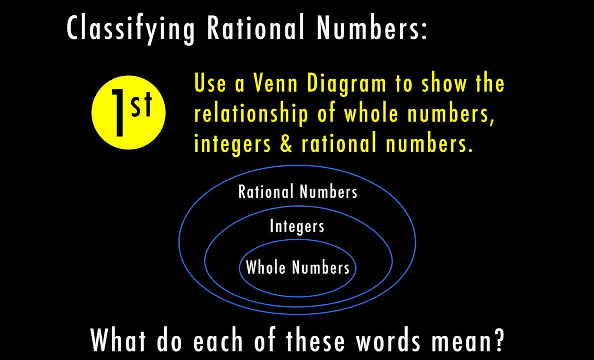 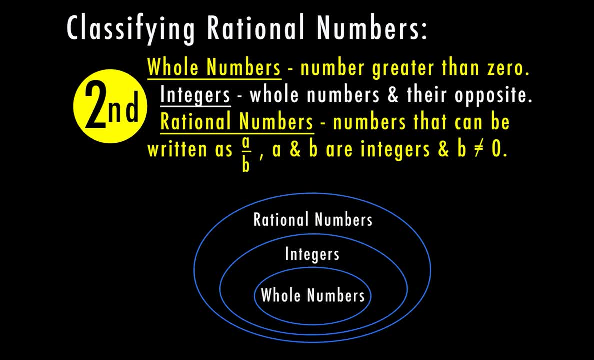 we have those categorized better. So what does each of these definitions or words mean? So we have whole numbers, which is a number greater than zero. We have integers, which are whole numbers in their opposites, and we have rational numbers, which are numbers that can be written as a over b, which. 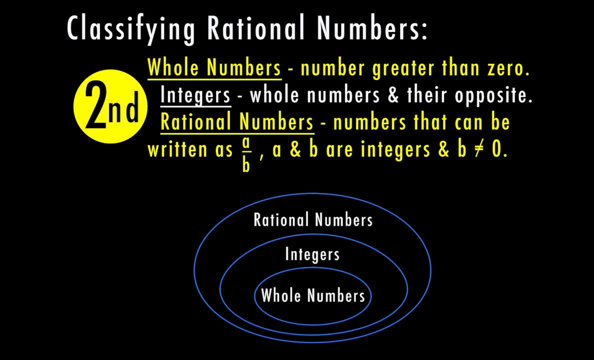 is a fraction where a and b are integers and b cannot equal zero, So the denominator can't be zero. Now, whole numbers means you have 1,, 2,, 3,, 4, and so on, all the way to infinity. An integer would. 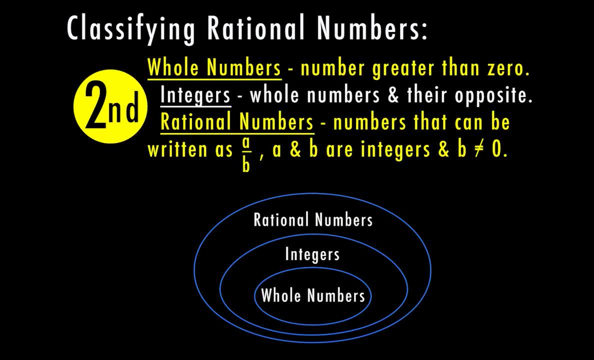 be 1,, 2,, 3,, 4, and their opposites, which is negative 1, negative 2, negative 3,, negative 4, and so on. A rational number is a number that is either a fraction, or that fraction can be written in a. 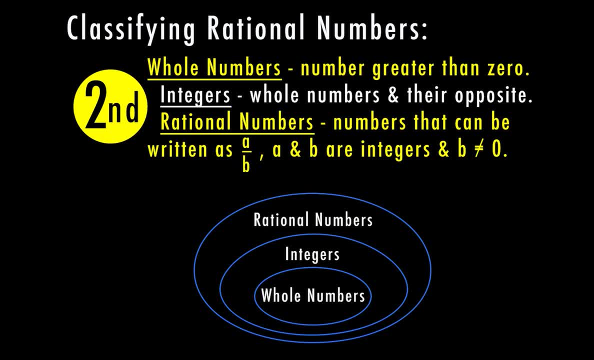 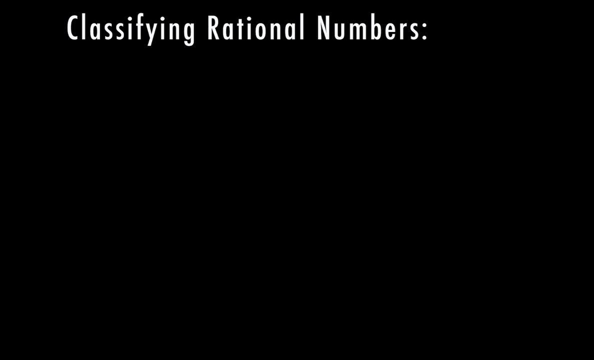 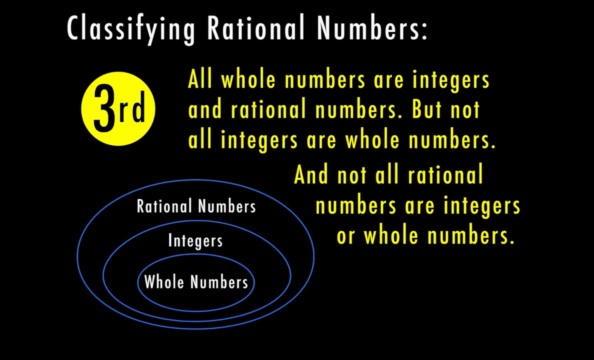 different form, which would be typically a decimal. So those would be the rational numbers as far as the outer ring. Now, rational numbers can also be negative, but if they're a rational negative number, they still only go into the rational number category. So for our third step here all whole numbers are integers and rational numbers, So all numbers. 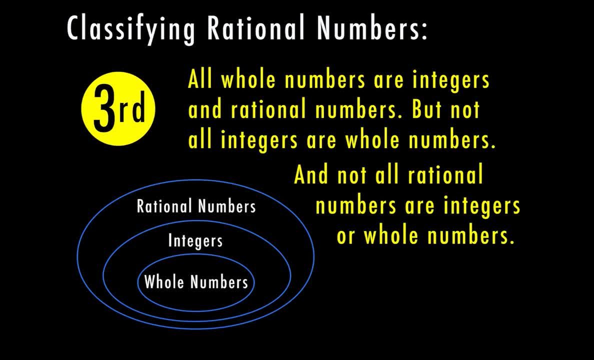 that belong in this center circle, the whole number circle, are also going to be categorized as integers and rational numbers. So a number can be in all three categories, or it could be in just two, or sometimes just one. Not all integers are whole numbers, so four is a whole number and it's an 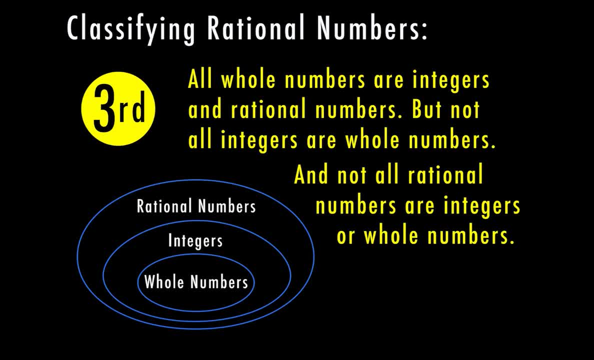 integer. So if you have a million numbers in your whole number it's going to be a whole number. Negative 4 is an integer but not a whole number, because whole numbers are not represented by negatives. Not all rational numbers are integers or whole numbers. 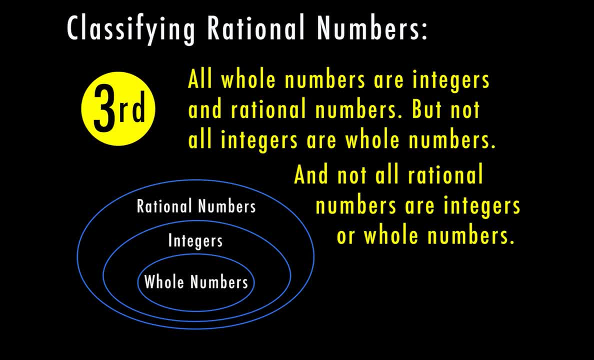 So if I have the rational number 3.4, or 3 and 4 tenths, that would be written either as a fraction or a decimal. Either way, that's a rational number, but it is not an integer and it's not a whole number. 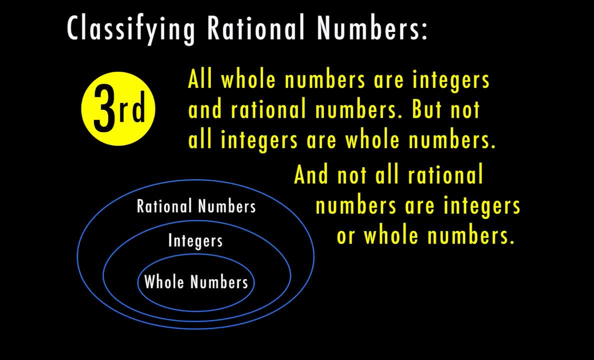 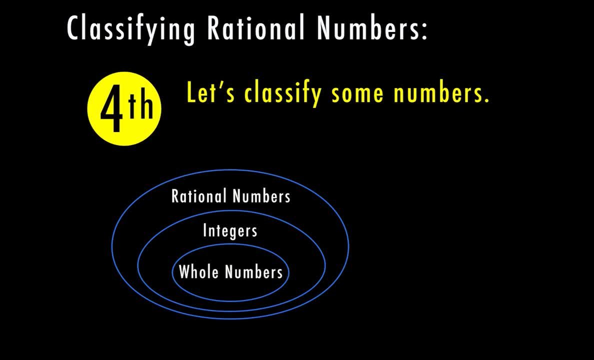 So what does this mean? Well, what this means is that we can go ahead and use this information to classify some numbers. So I have a list of numbers here, So let's go ahead and put them into their categories. So the number 4 is a whole number, so we're going to put that number here in the whole number category. 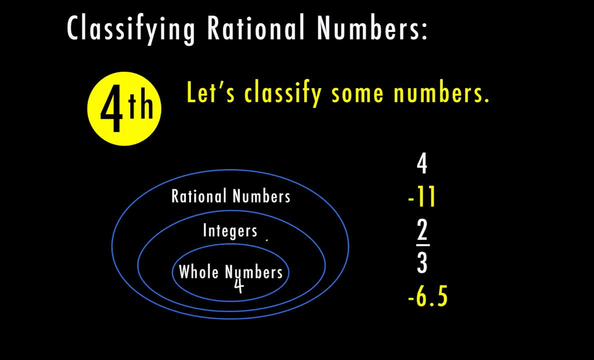 The number 4 is a whole number. The number negative 11 is an integer, so I'm going to put it here in the integer category. The number two-thirds is a fraction, so it's going to go into the rational number category. 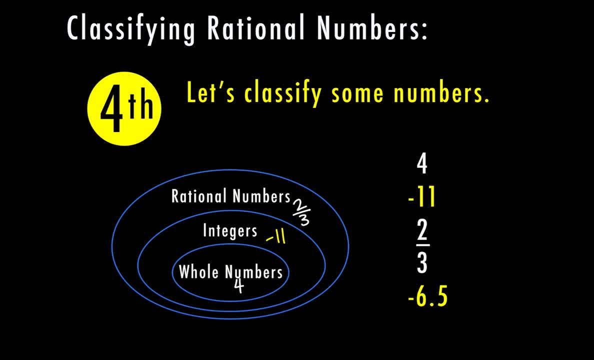 And then the negative 6 and a half or 6 and 5 tenths is going to go also in the rational category. Now, negative 11 is an integer. It's also a rational number. Two-thirds is a rational number. 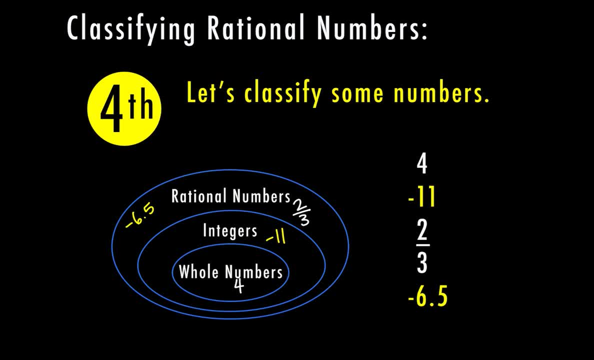 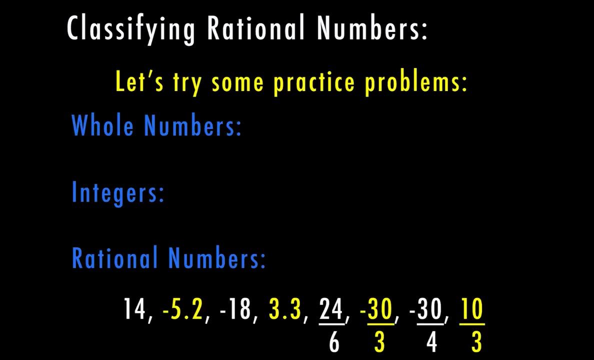 But it is not an integer or a whole number. However, this 4- that's a whole number- actually is all three of these when it comes to representing numbers. All right, so let's go ahead and practice and put some of these numbers into categories. 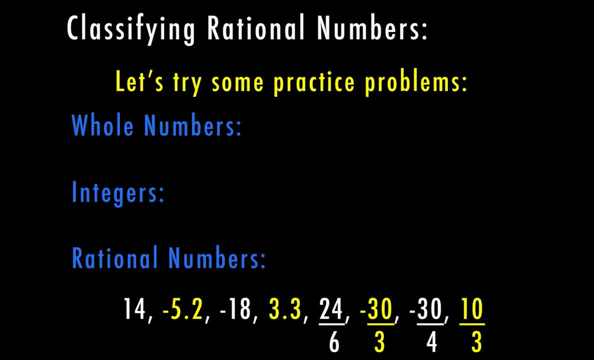 So down at the bottom I have a list of numbers, And then to the left side we have each of our categories listed. So we're just going to list them out into each category And then we're going to start with the ones that they belong to. 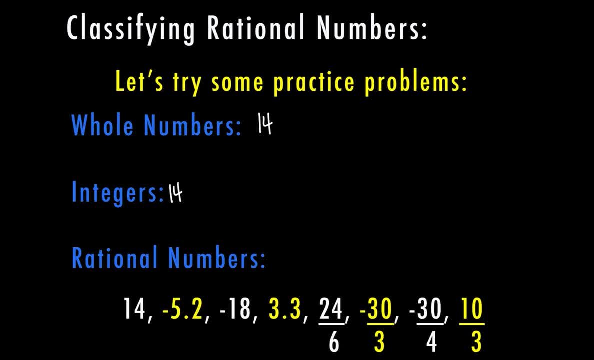 So the first one we're going to start out with is 14.. And 14 is a whole number. It's also an integer And it's a rational number, So I'm going to mark that one out. Now we have negative 5.2, or negative 5 and 2 tenths. 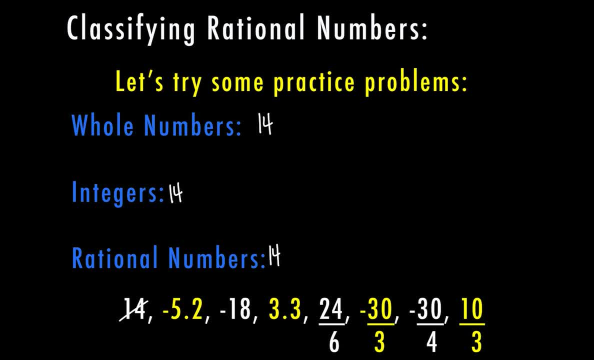 Well, it's negative, so it could be an integer, But it's not a whole number, So it's just going to fit into the rational number category. The third one we have here is negative 18.. 18 is a whole number, but negative 18 is not. 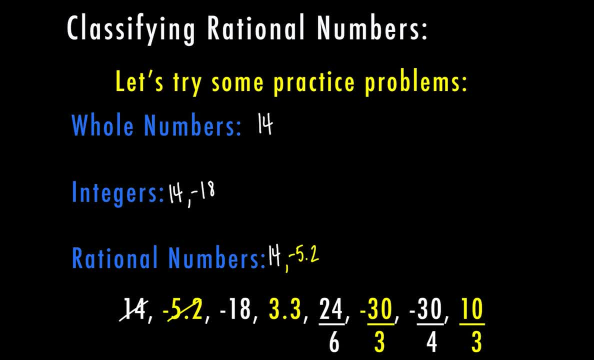 So it's just going to fit into the integer category and the rational number category. Next we have 3 and 3 tenths. Well, 3 and 3 tenths is a decimal, or it fits in that A over B form. 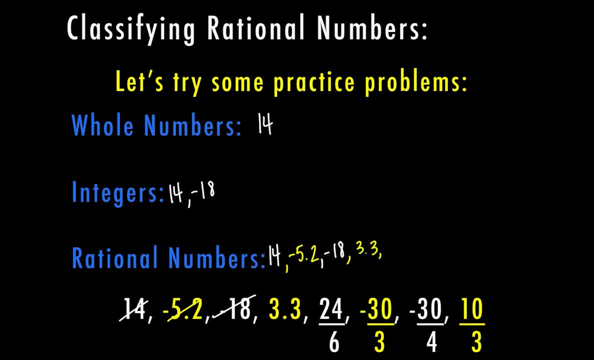 So it's just going to be a rational number. Next, we have 24 over 6, or 24 sixths. Well, if we were to divide 24 by 6, we get 4.. So this actually reduces to the answer 4.. 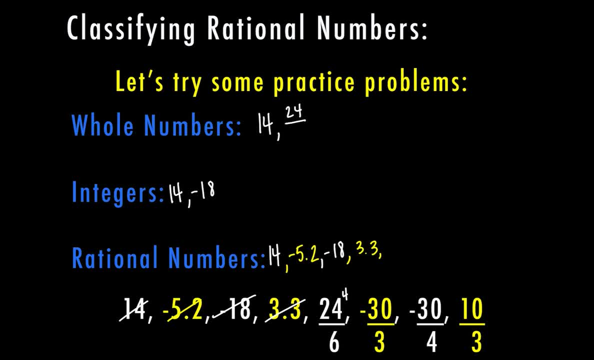 4 is a whole number, 4 is also an integer And 4 is a rational number. So ones like that look tricky because it does look like just a fraction, But if you actually reduce it or simplify it, you end up with all three categories. 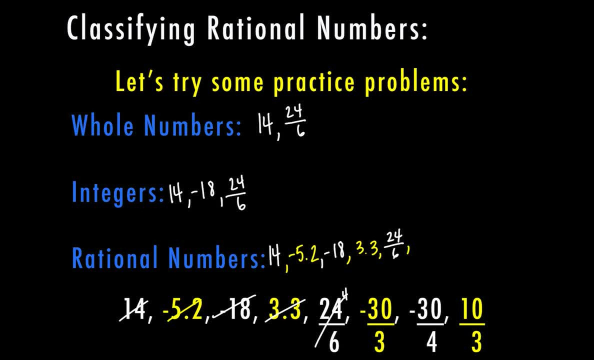 Negative 30 over 3, this is another one. I can go ahead and reduce or divide it. So negative 30 divided by 3 is a negative 10.. So this is going to go into the integer category and the rational number category. 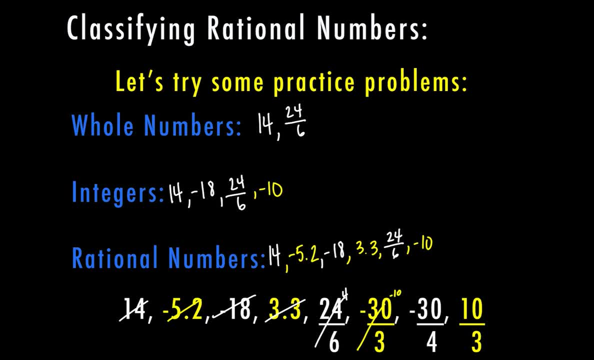 And we haven't learned how to divide by negatives yet, but we're still going to use it as an example. Negative 30 divided by 4, this one does not go in evenly. 4 goes into 30 seven times. And then I have 2 fourths or 1 half left over. 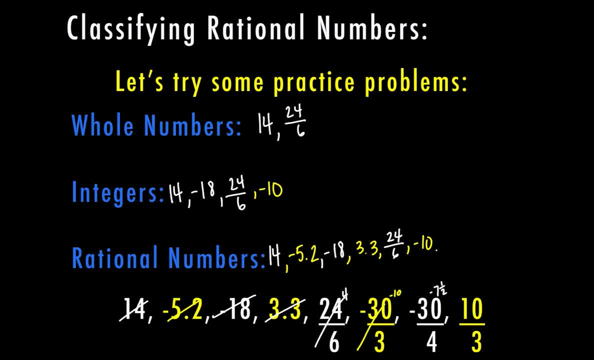 So this one is a negative 7 and a half, So that one just fits into this rational number category. And last we have 10 divided by 3, which goes in 3 and 1 third. So this is also just going to be. 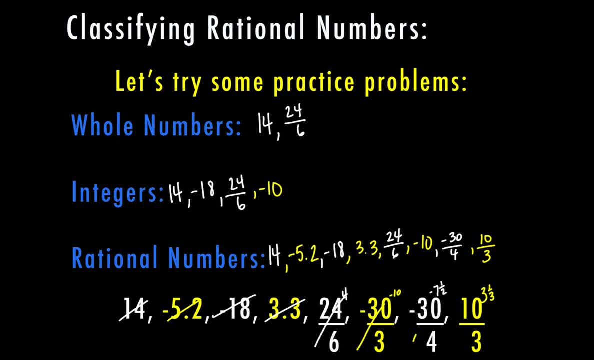 a rational number. So we can take each of these numbers and we can put them into all the categories that they belong to. And, if you notice, there's more rational numbers than integers and whole numbers, And that's because all whole numbers are integers and rational numbers, but not all rational numbers are also whole numbers.